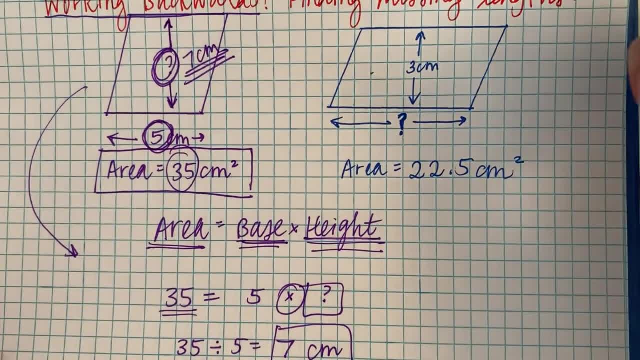 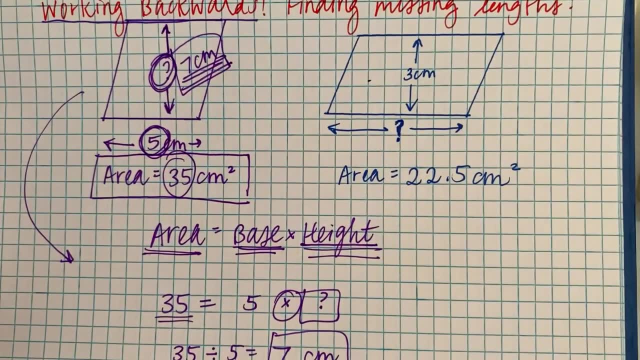 measurement of length. so it's just centimeters. so that would be your answer. that would be the height of that parallelogram. all right, so if you want to try to find the missing value on this next one on your own, go for it. I'm going to go ahead and do that, and then I'm going to go ahead and do that. 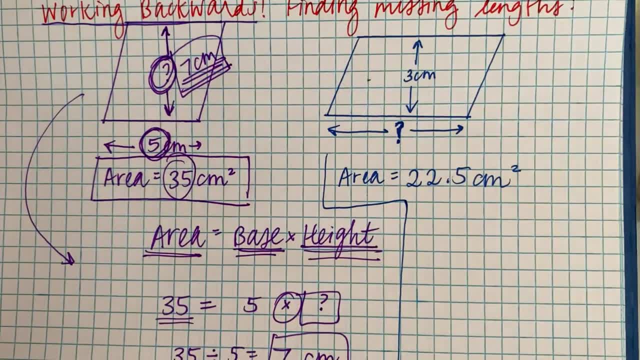 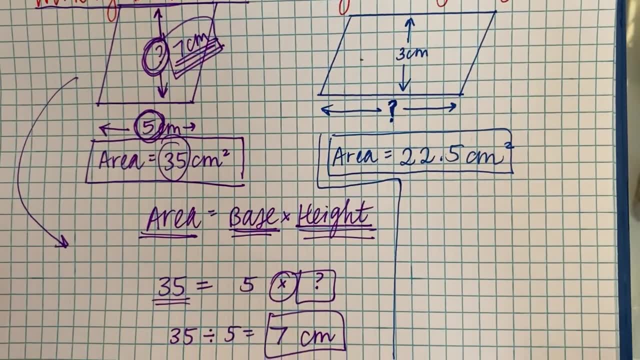 and then I'm going to go ahead and do that, and then I'm going to go ahead and do that. otherwise, pause the video, otherwise we can work it out together. so this one here. the area is given to us as 22.5 centimeters squared, so we're given the 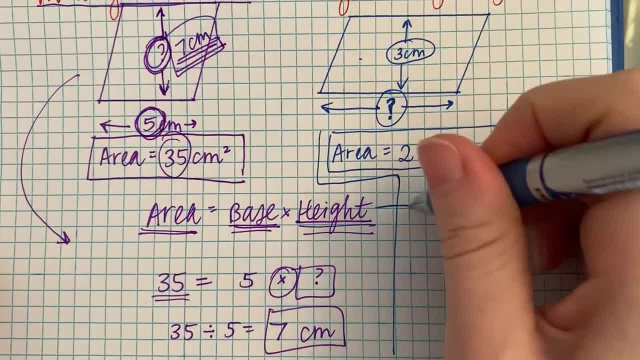 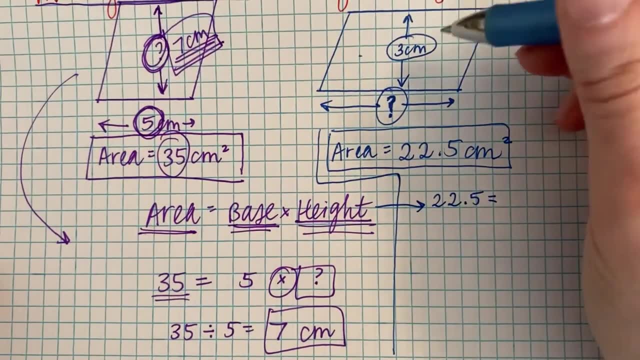 height this time, and we're looking for the base. so, if you want to, you can fill this formula in as well. area equals base times height. so 22.5 is equal to the base, which we don't know- question mark times the height, which is 3. all right, so? 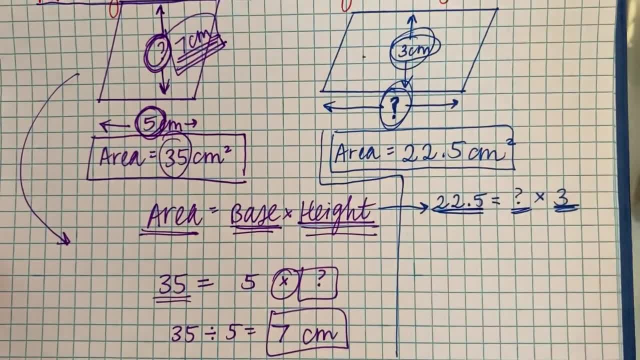 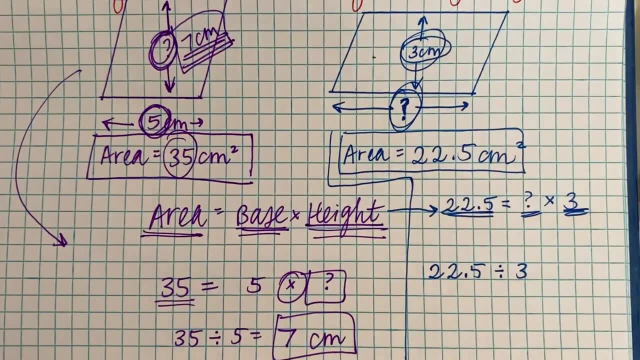 we need to figure out what do I multiply by 3 to get my area of 22.5? or we could think of that as working backwards, 22.5 divided by 3. okay, just working backwards. so 22.5 divided by 3. 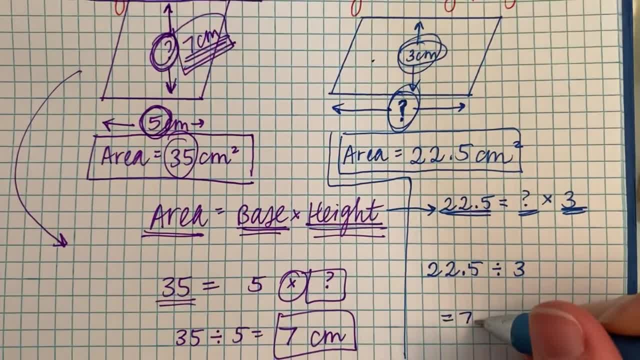 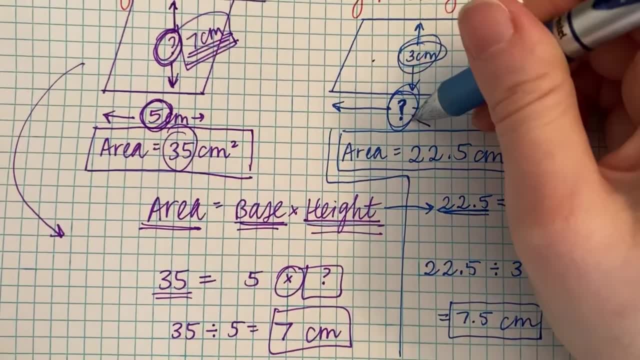 would give us 7.5, and again, this is a unit of measurement of length, so we would just use centimeters to describe this distance here. so our answer is 7.5 centimeters. 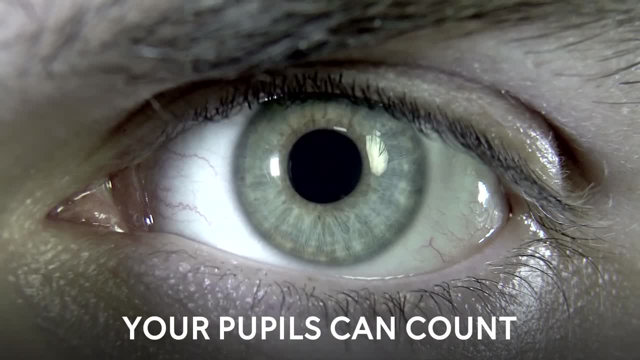 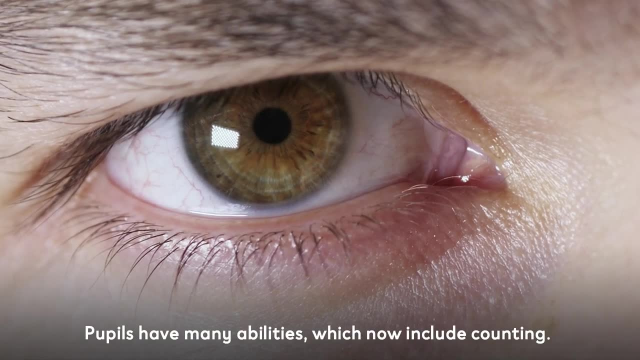 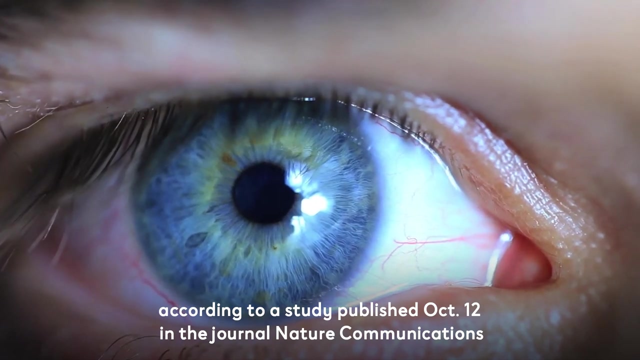 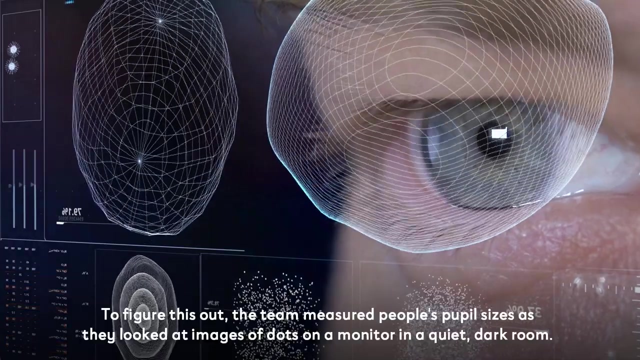 Your pupils can count. Pupils have many abilities, which now include counting. According to a study published October 12th in the journal nature communications, People's pupil sizes change depending on the number of objects they see around them. To figure this out, the team measured people's pupil sizes as they looked at images of dots on a monitor in a quiet 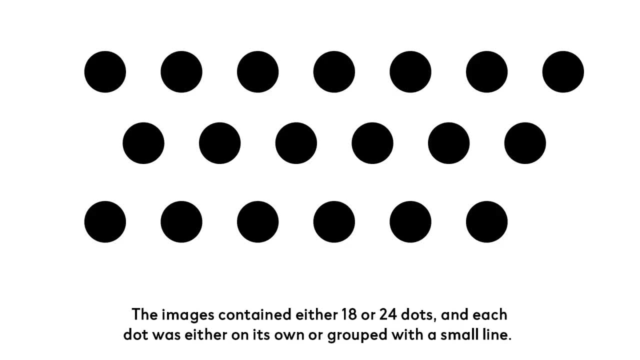 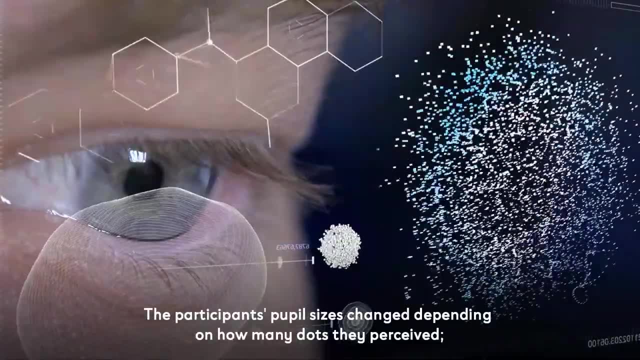 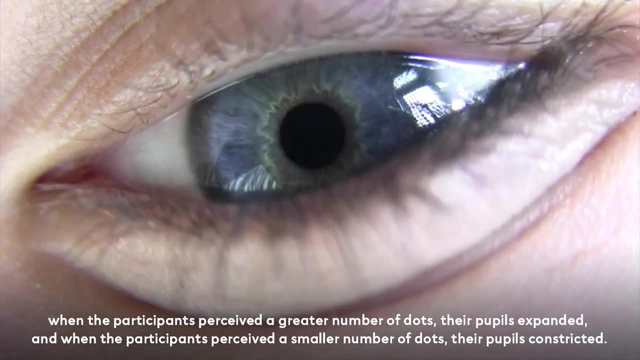 darkroom. The images contained either 18 or 24 dots, and each dot was either on its own or grouped with a small line. The participants pupil sizes changed depending on how many dots they perceived. When the participants perceived a greater number of dots, their pupils Expanded. and when the participants perceived